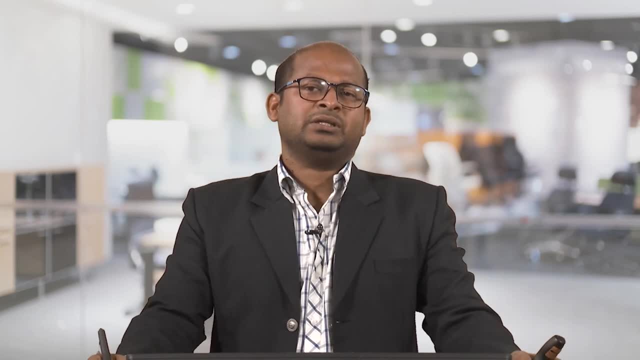 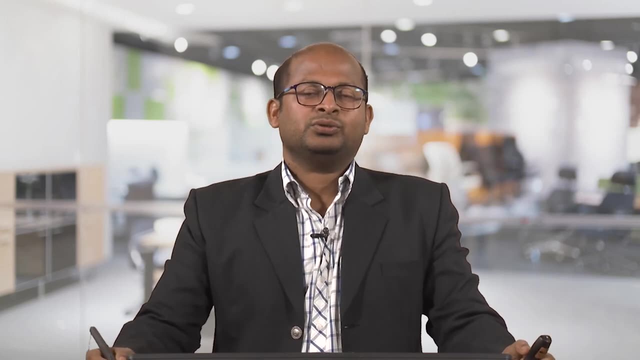 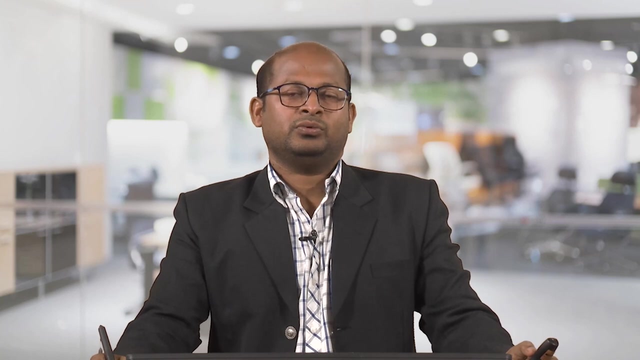 Reactor has many problems, means once we design the reactors. many way we can design the reactors So for our to purpose, the reactions. So once we have that particular reactor, so reactants, once we charged, so reactants go inside of the reactor through the inlet. 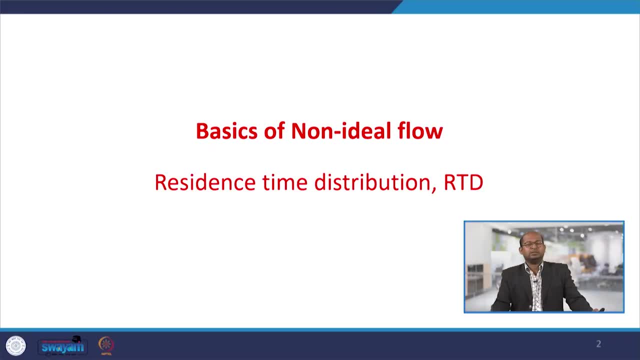 of the reactor Once it is passed inside of the reactor. so if it is small reactor it is fine, but when it is So industrial scale, large reactors is there and large quantity of the reactant that is feeding through that feed inlet. And if it is one component or multiple component of 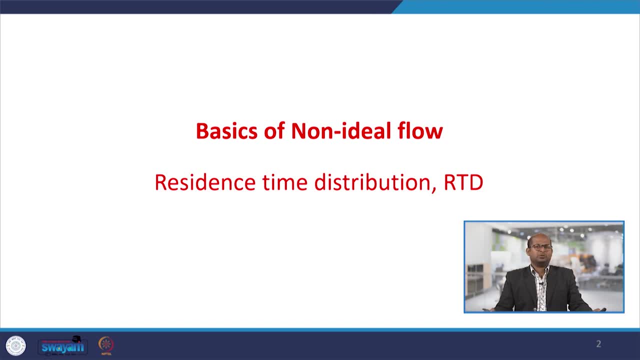 the reactants are there, so then their distributions means how they are flowing inside of the reactor. that is very important. Means the nature of the reactant once it is enter inside of the reactor, So how they are behaving there. So means how long. means if we know the volume. 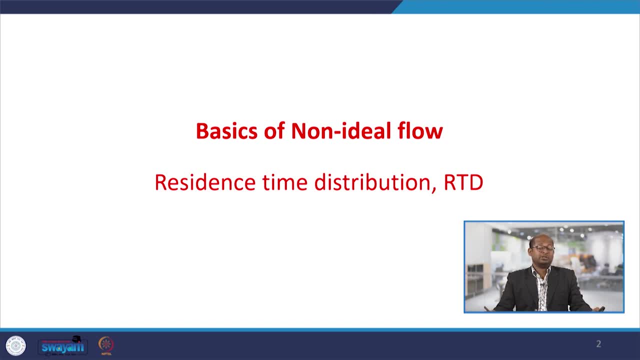 of the reactors, volumetric reactors, volumetric flow rate, that is the fixed, then residence times or space time, that is the tau, that is the fixed for all component, whatever it is entering in the reactor. But if, let us say, the reactions, A is going to A plus B, A going to this, C plus D means 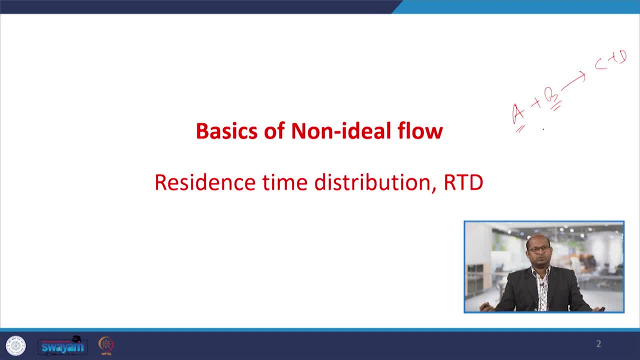 here reactant A and B is there. So once these two reactants come in contact, then only reactions will proceed. So mixing is very important in between two and if reactant is passing through these reactors, let us say: A is going, B is also going, but A is taking less times. 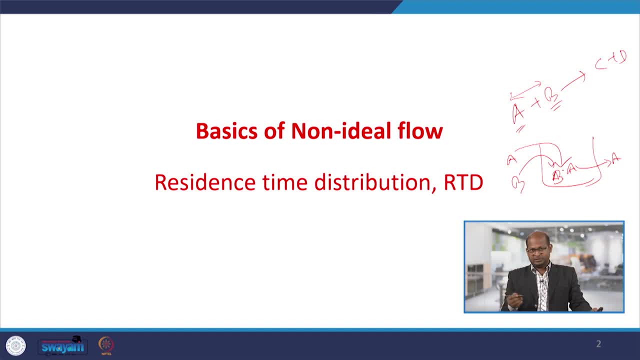 it is leaving from the reactors but B is present there. so B will not interact with the A, so then there would be reactions. would be means there is no possibility of reaction, So they will not interact with the A. So B will not interact with B. then they will. 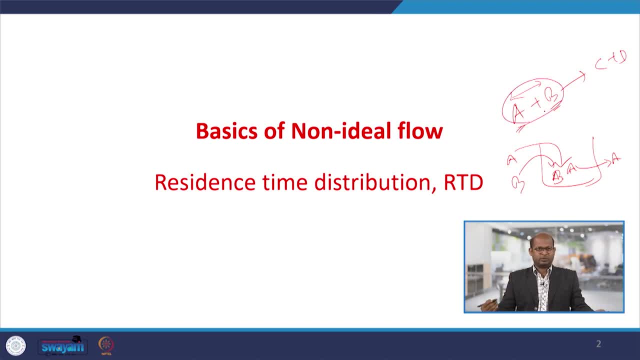 both come in contact. in the right environment means temperature, pressure, catalyst contact. So then the reaction should be proceed. So means somehow some anomaly is there once it is entered. So sometimes we get low concentration, low conversions, sometimes we get high conversions. 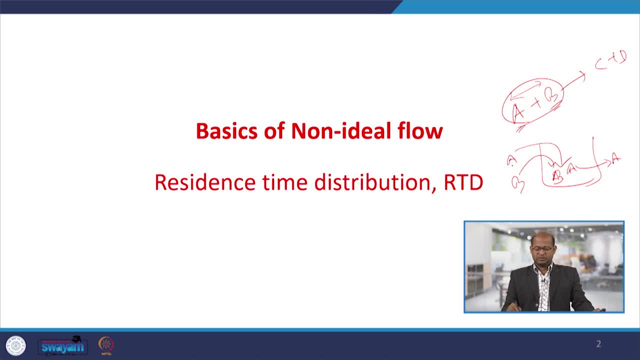 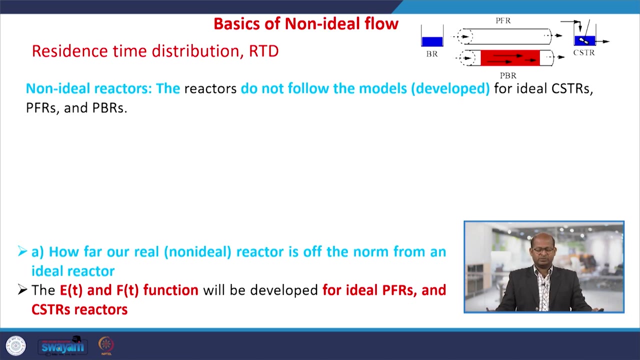 means fluctuation is there, So that is due to the distribution or residence time. distribution or the times they spend inside of the reactor May be reactant to reactants are different and that may be due to the fault of the reactors that we have designed. So that nature means 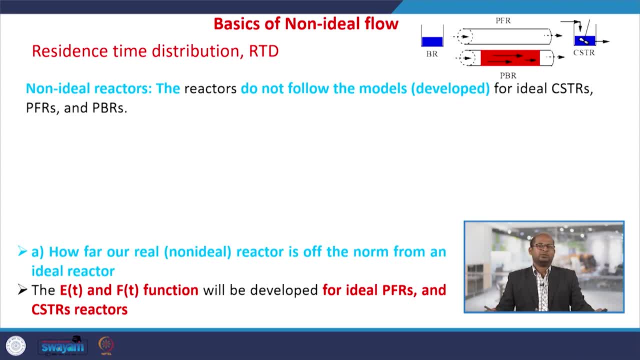 up to means always, whatever the reactors we designed or we fabricated, that is real reactor. So how the real reactors is deviated from the ideal reactors when non-ideal is coming from, with that ideal also is coming. Non-ideal means that is the real reactor, that is does. 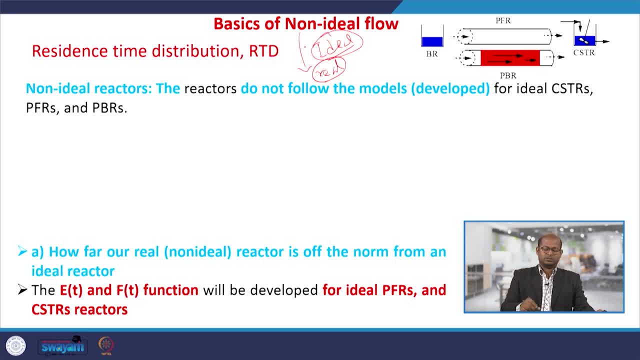 exist, and ideal that is not exist Means Whatever the reactors that we develop or design, fabricates, that should be close to ideal. If it is far away from the ideal, that is not acceptable from the industrial point of view for the reaction if you want to conduct So, therefore, always that should be close. 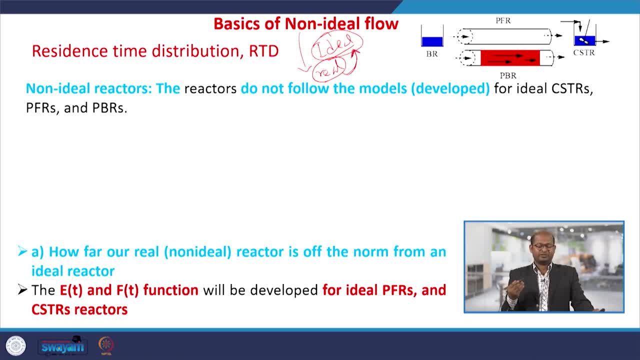 to ideals. not exactly ideal is not possible. perfect reactor So close to react ideals, the reactors we can develop. So these are the things means residence time distributions we have studied against will study it here. sense in the few lectures will get an idea about various type of models. theoretical models have been developed, So that will discuss. 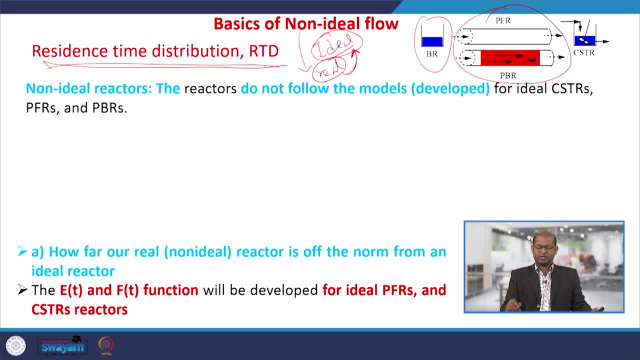 So these are the reactors we know. So this is plug for reactors. this is the Packweed reactor, this is CSTR reactor. So these are very common reactors. In these particular reactors, non-ideal flow natures we will discuss. that means the residence time distribution. 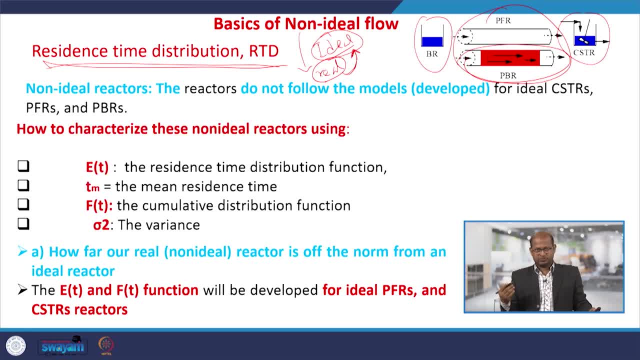 we will discuss. So in this particulars means the reactors We have to want to, means study. So this is a same reactor that have difficultقing быстрere. So we have to try the Silver warp reactor. What you call D tang is mean in the death reaction and never in fusion reaction. In the photo you have the 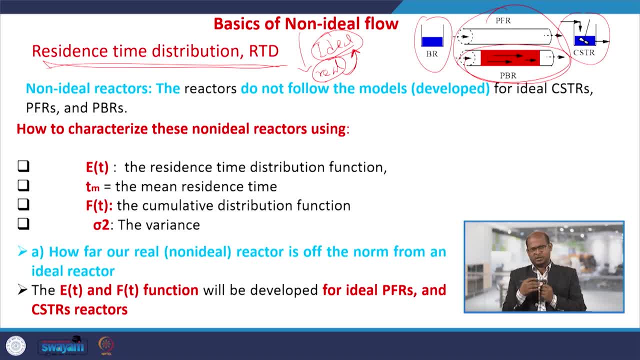 study want to characterize that particular reactors. what are the deviation? is there? up to what extent it is deviated from the ideal? So that we want to check means whether our, the reactors we have, design is perfect or not that is suitable for that particular. 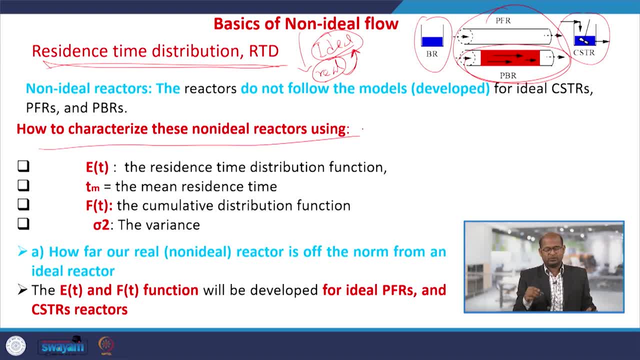 reactions or not. So, then, to characterize this non-ideal nature of the reactors. so Et, we have to know, Tm is, we have to know Ft and sigma square, that the things we have to find out. So what are these components we already have? 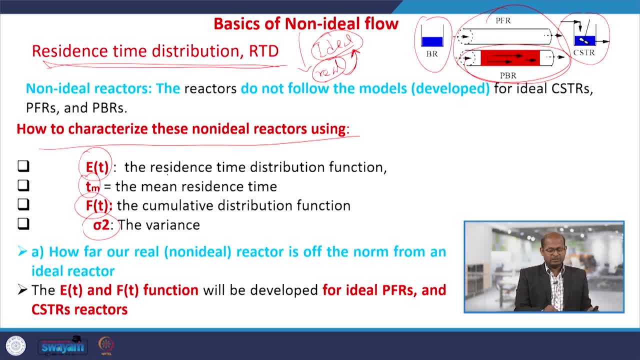 studied in UIG courses. again we are repeating here. It is the residence time distribution functions of that particular components or reactants that we are feeding inside of the reactor. that functions. residence time distribution functions have to find out for the reactor. we have to check that. we have to test that Tm is the mean residence time that component. 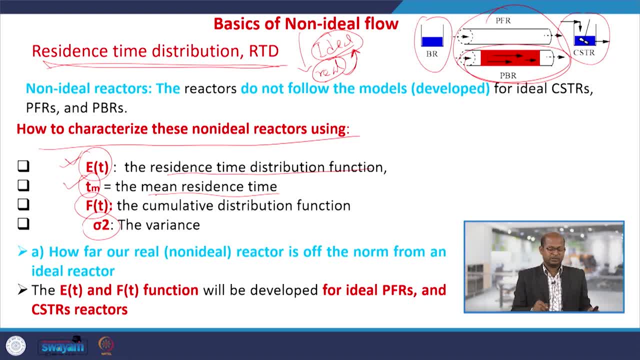 is present or passing through these reactors, the mean residence times of individual component or the reactants. We have to know cumulative residence time, distribution function and sigma square. that is the variance we have to know. So means the to characterize this reactor, basically our reactors, is of norm from an ideal reactors, so by this way you can find out. 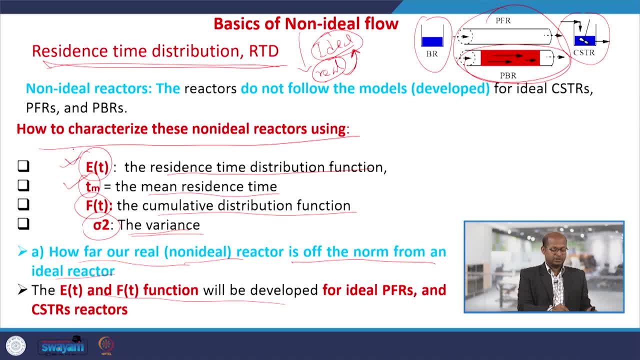 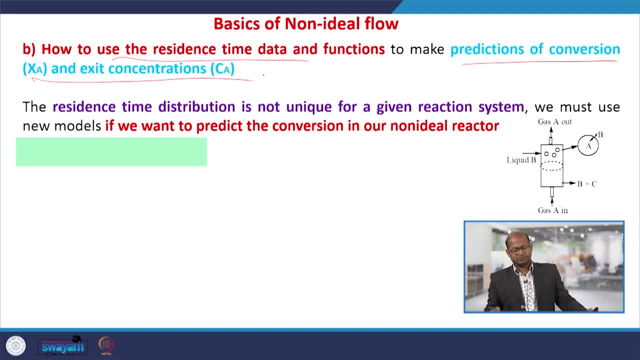 And second is: once we know these are the components, so using those components we can find out, means predict, we can predict the conversions and exit concentration. means, once we have, let us say So, these are the components that we have to calculate these reactor we have. So here, 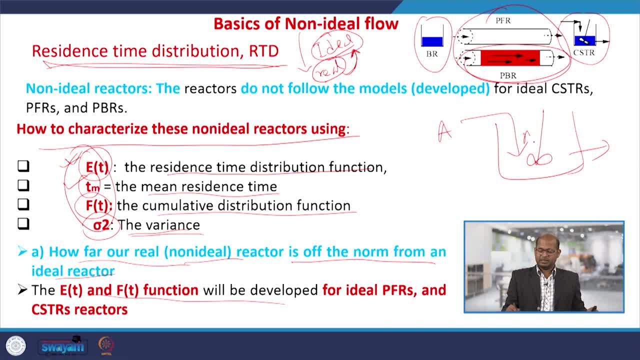 we are conducting any reactions. A is coming here. So if it is 10 milliliter volume of the reactors, it is small volume of the reactor. V equals to 10 milliliter. So here conversions means C, A, initially. let us say 100 mole per dmq. we have given charged and at the end of 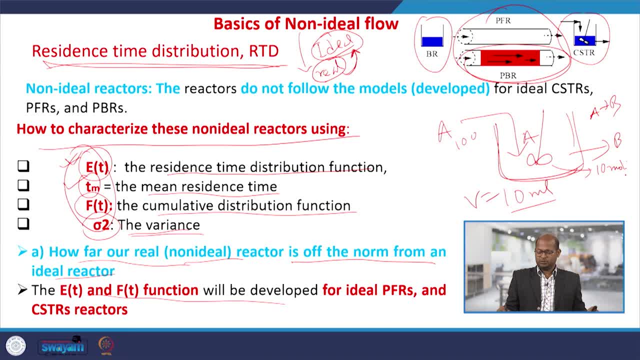 the reactions. let us say, 10 mole per dmq. we are getting So some of the components. we have to understand that. So we have to understand that these are the components that we have to know. So here, we have to understand that. So these 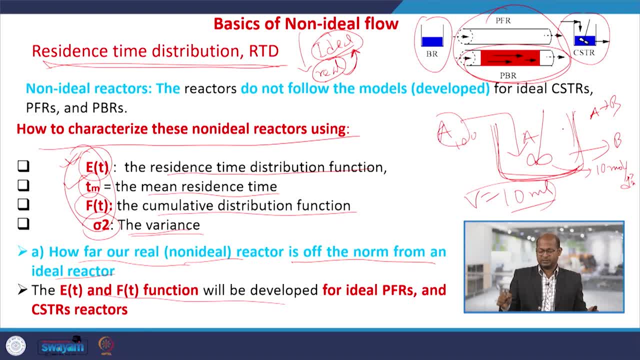 small reactors, small quantity of the reactants, we can pass here easily. we can measure, we can characterize these reactors, quantify we can do. but when large scale reactor is there, so here volume was 10 ml, here volume let us say 1000 liters. so if we check these reactors means then we have to. 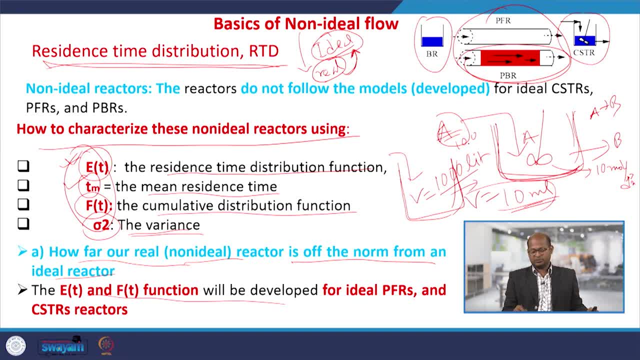 conduct the reactions. so but if this reactant is very costly, let us say thousand rupees per gram, let us say or per kg, so very costly, so too much. means reactant you have to pass to check that things, but this is sometimes is not possible. so means to the reactors for industrial design. 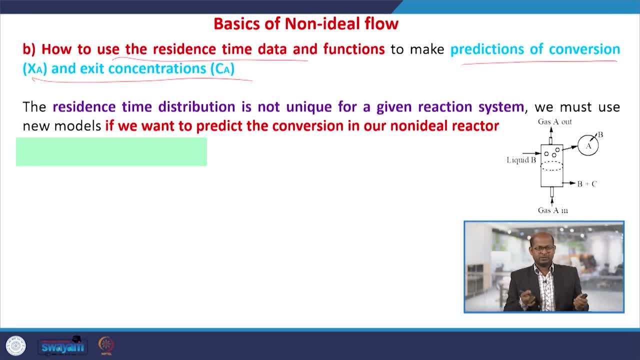 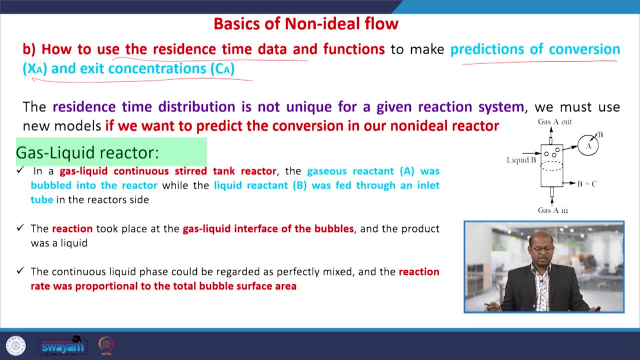 you have to check that. so, for this is the basic purpose of this rtd study, or residence time distribution study, so by considering, instead of reactants so we can put something inert materials, so by that we can check that. that will come discuss later. so here's the residence time distributions, why it is required. so to predict the conversions of a. 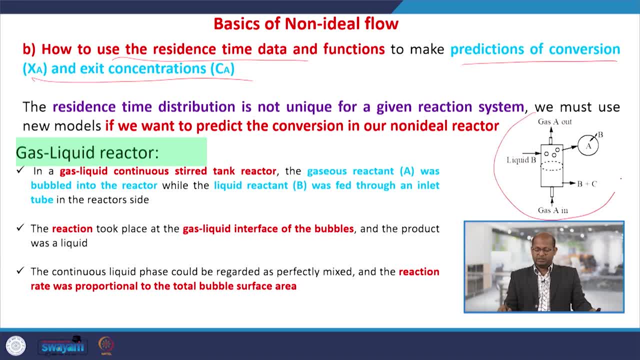 non-ideal reactor, so that we basically discuss here and then we go for that. so let's say, gas liquid reactor contactor is there, or sludge type reactors or other type of reactors is there? in that case, two phases are there. reactant is a is. 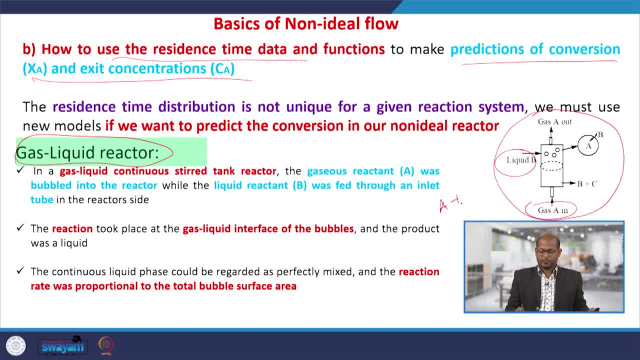 the gas and liquid component. a is the gas and b is the liquid. so these are the reactants. so b is passing from the tops and a is passing from the entering, from the bottom of the reactor in the form of bubbles, gas bubbles. so a is leaving this way and b is coming after reaction this way and 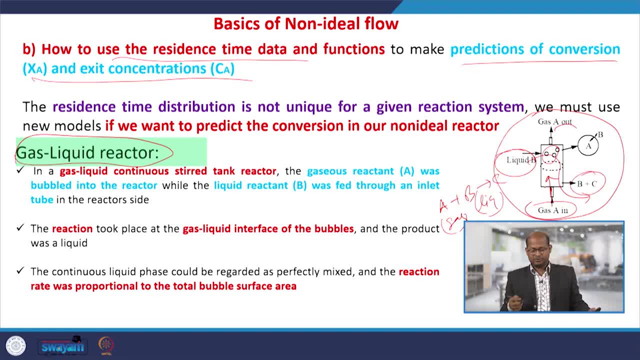 product formation is there, c is is with b, c if c is the liquid, then both will come from the downs. so here's bubble formation says bubbles, and here's the interface. a and b is there, gas and liquid. their reactions will take place. okay. so here's the residence time distributions, why it is important. so here the 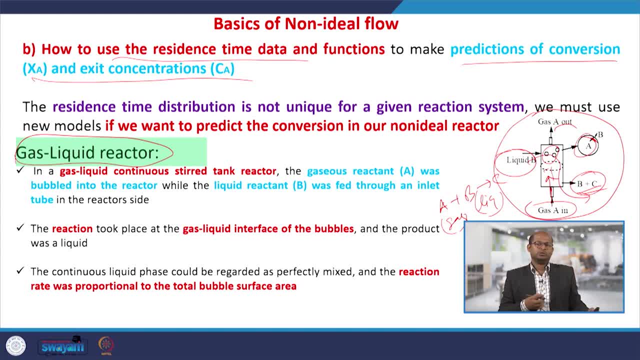 bubbles that is coming from the bottom to the top, so it resides different times inside of the reactors. its size also is different bubbles diameters, meters and so on- so that is the reason why it is important. so here the bubbles that is coming from the bottom to the top, so it resides. 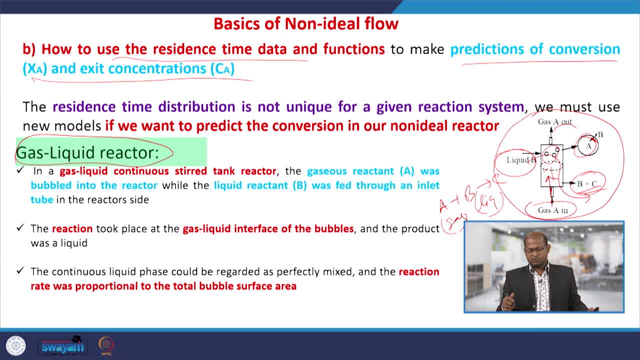 maybe smaller, larger in different type of there. so therefore the interactions are in contact interface. contact in the bubbles would be difference. therefore overall conversions, distributions would be different. concentration, that is the coming out, exit concentration here, exit concentration of the b is coming different and that would be difference, means actual how they. 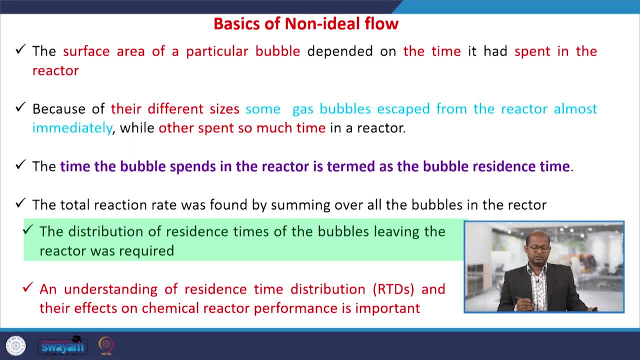 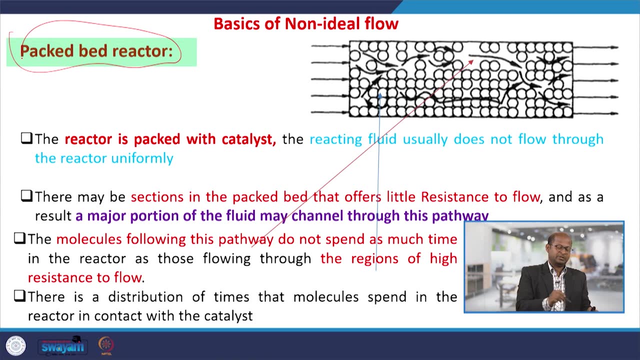 are behaving inside of the reactor, so why they are changes that. if you want to know, so then this rtd to check the reactors so to understand the residence time distribution and their effect of the chemical reactor performance we need. similarly for a packed reactor is also this: 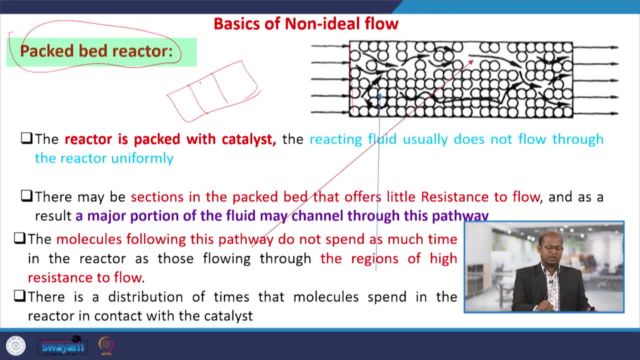 is the packing material? is there in the packed reactors? we usually put solid catalyst here and then reactant is passing. a would pass through this bed. catalyst bed is there? okay, so when reactant is flowing, here means some void spaces. are there are some molecules? uh, without interacting with the 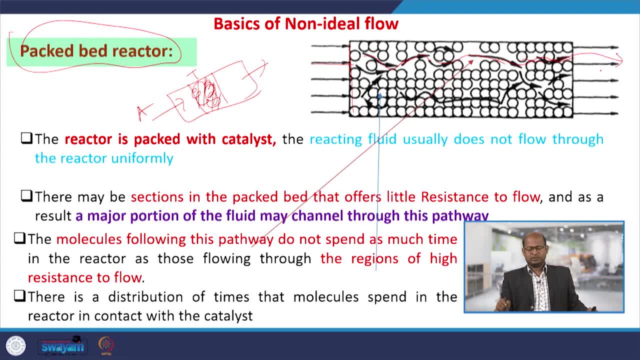 catalyst surface they are leaving from the reactors. it takes very less time. if there are some molecules spends longer period of times, they are not getting space to leave from the reactors, so remain there inside means accumulation should be there so and few interacted with that catalyst surface and leaving from the reactors after reactions. so then, these are the things of 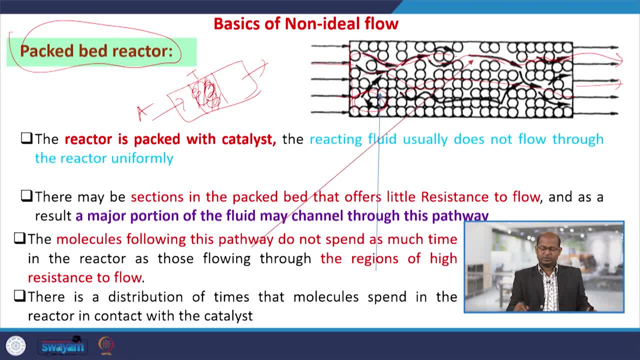 the packed reactor. so, uh, this type of means when reactants leaving without interacting with the catalyst surface. if it does not interact with the catalyst surface, there would be no reactions. therefore, this type of things means without interacting is called channel, okay, channeling. it is called okay without reactions. or reactants with the surface of the catalyst it is leaving. 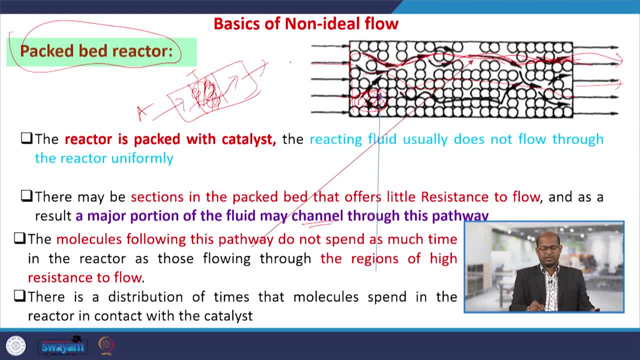 so this is called channeling and means once reactant ca 0 is there, here is ca, so without reacting. if reactant pass through the reactor then conversion should be low. okay means all the reactant does not take part in the reactions, so few molecules take. 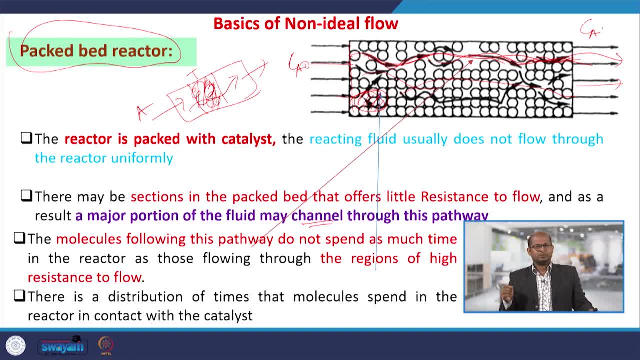 part in the reaction. so therefore, so that is not acceptable. when we design a packed reactor, so we expect that all the reactants should pass through the catalyst bed, interact with the catalyst, take part in the reactions and then it would leave from the reactors. okay, but in real case, or the 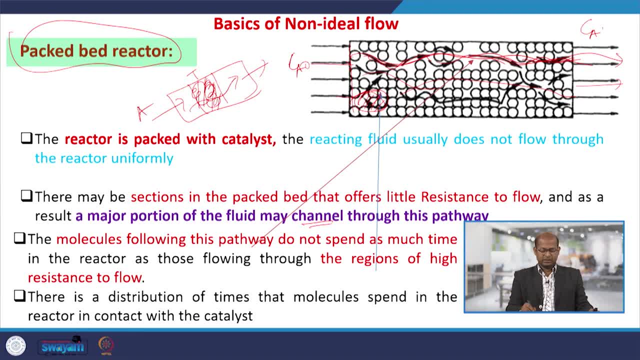 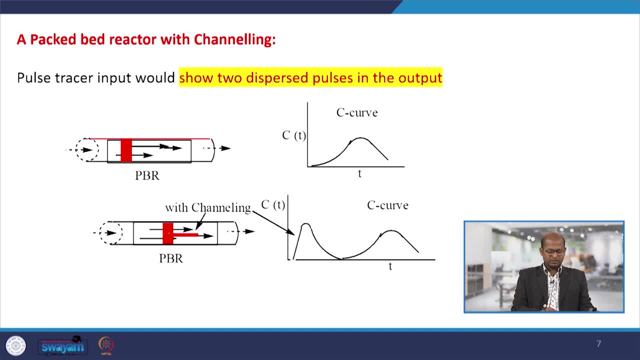 real reactor. that does not happen. so sometimes channeling is there, sometimes accumulations is there then. so overall performance of the reactor should be different. so this is the channeling, so it leaves before the times. so then, what kind of concentrations? or if channeling is there, so it is the called c curves. what is the called c curves that you 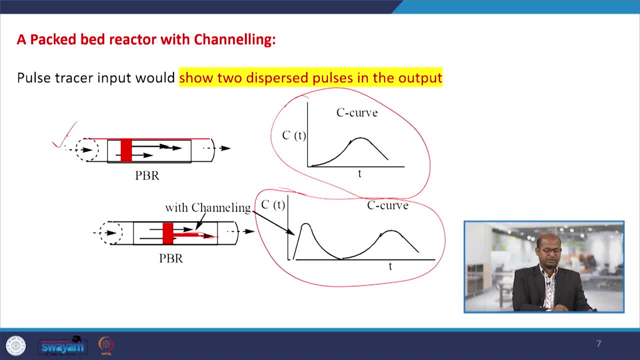 already have studied. and c curves: if reactor we have designed perfectly packed reactor, so then this type of natures of the concentrations means reactants. if we pass, let us say, ca, ca concentrations, it would be 0 in the initially, and then it would go maximum and then decrease and then so all the 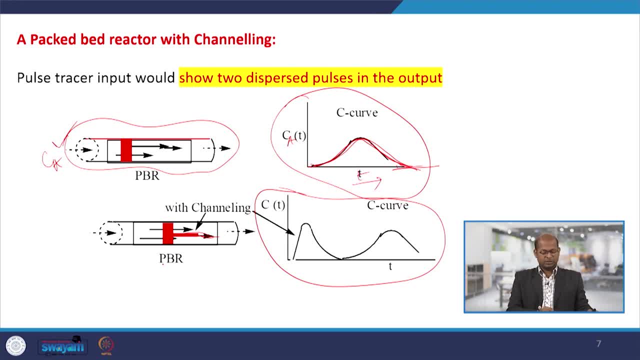 molecules leave from the reactors with the different times. so similarly, if channeling is there, so then suddenly few molecules will come out and then again it reads to the zero or down, and then again reach to this. so in addition, this is the natural and this is also expected. so but 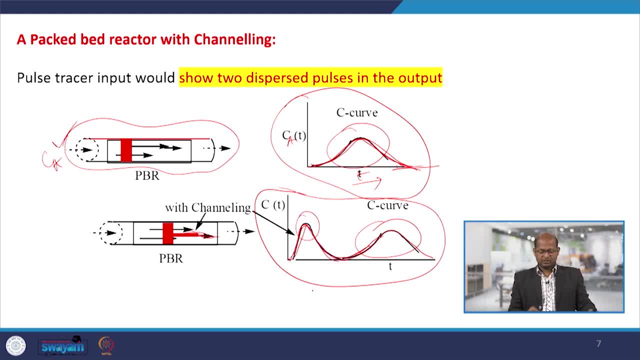 this is coming, so this type of bump is coming. that is, or may be different type of also may be coming this type of, so this type of bump is due to the this type of channeling so very fast. the before means maximum times, or tm is the maximum times may be up to this: 0 to, let us say, 10 minutes. but 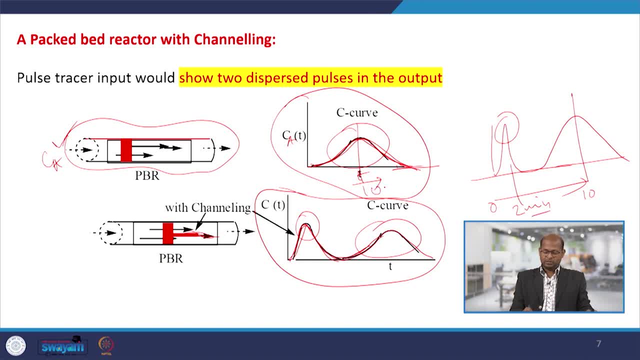 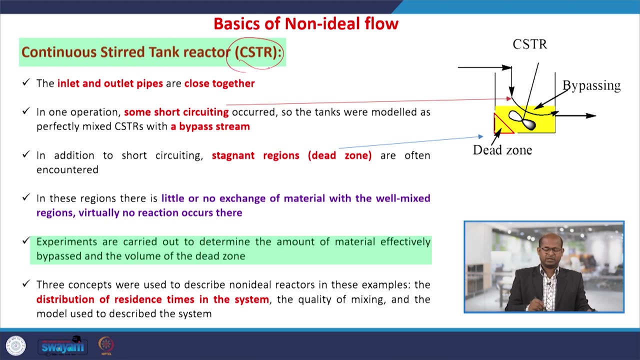 0 to 2 minutes. few molecules are coming here. also 10 minutes or maybe 12 minutes, whatever. so before time that molecules is coming or coming out from the reactors. so these are the things means study so that we will discuss later. so similarly continuous start tank reactor is also there in. 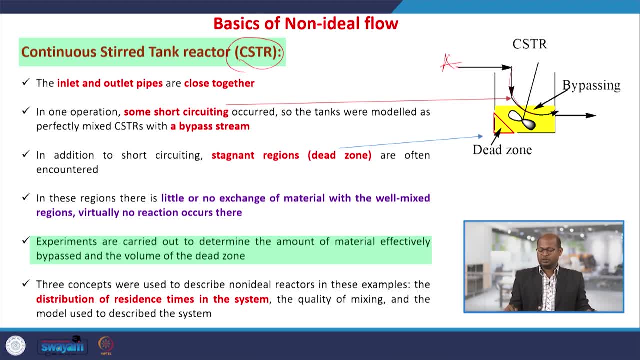 that case also reactant is passing here. so if outlet we fixed here, so then reactant molecules without mixings or taking part longer period of times it may leave from the reactor. this is called bypassing means. here a particular space is there within that reactant molecule spent that may be. 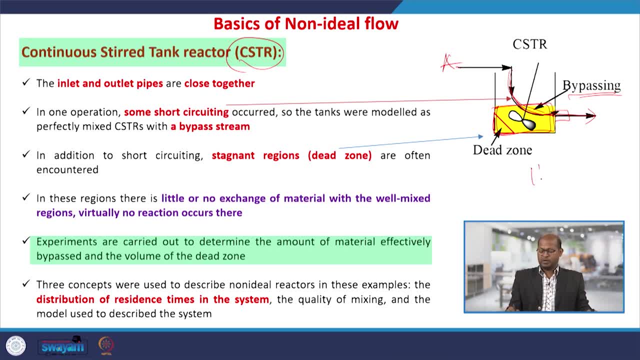 you are expecting, whatever the molecules is entering, one hour that should spend inside of the reactors, but few molecules following this pathway. it is leaving in after 30 minutes. so this is called staying very less time. so then conversions, yield, selectivity would be different and few molecules at this particular space. remaining for longer time does not take part. 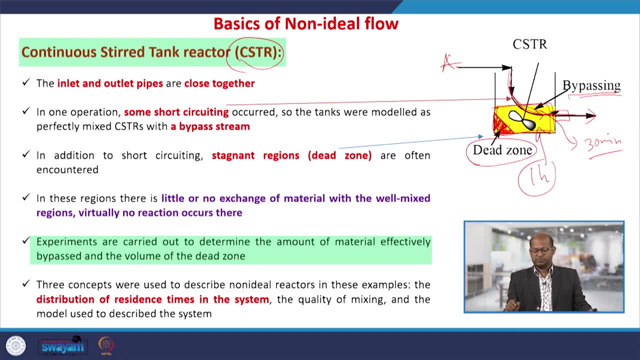 in the reactions. this is called dead zone, so instead of one hours they remain inside of the reactor 1.3 hours. so then several performance ca and ca naught. so based on that we can get ca naught minus ca by ca naught. so here ca is different, concentration would be different due to this. so therefore, 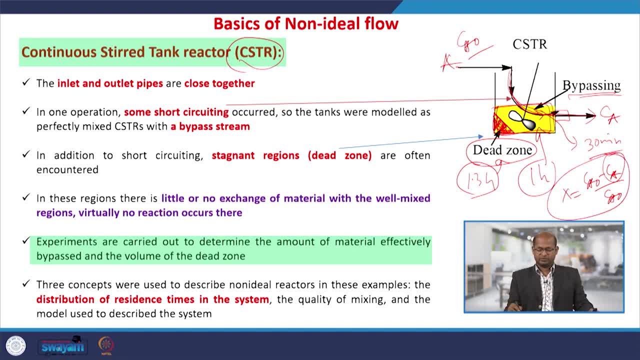 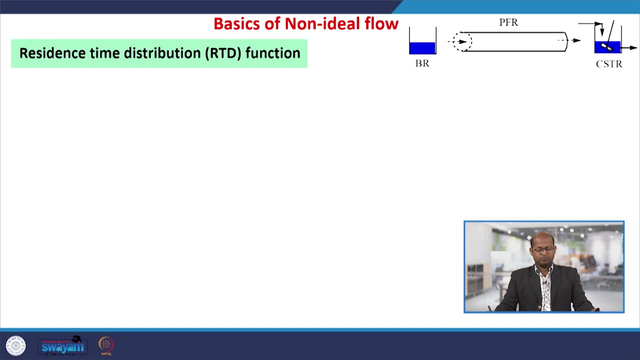 some performance or conversions of the reactor should be different. so if we, unable to design the reactor not perfectly, want to design the reactor perfectly, but if it is not possible, in that case this type of problems may appear and we have to address those things. so then, residence time distribution functions, that is rtd, so it is important. so we have batch reactors. 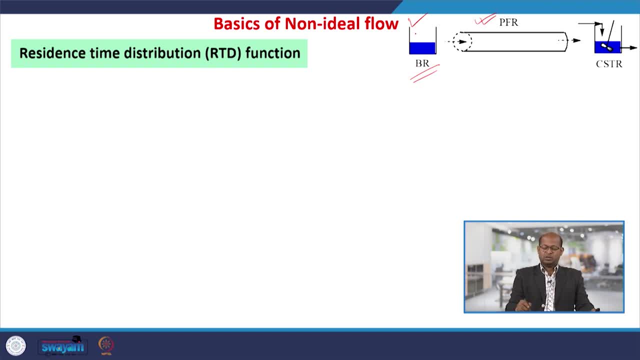 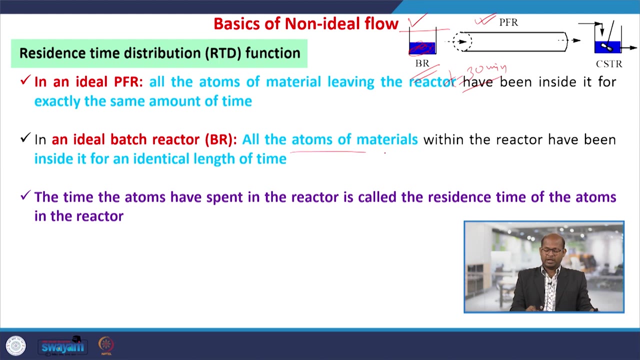 we have a plug for reactors in batch reactor. so let us say: all this is the reactant molecules. we put inside of the reactors and spent 30 minutes and after that we collect all molecules together. then batch reactors. all atoms or materials within the reactors have been 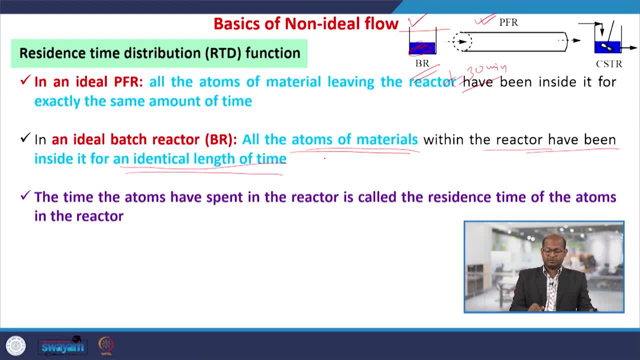 inside having identical length of times, that is, 30 minutes. let us say t equals to 30. i said so. all molecules spending same time. so then batch reactor is an ideal reactors. similarly, plug for reactors. all atoms or materials leaving the reactor have been inside for the same exactly. 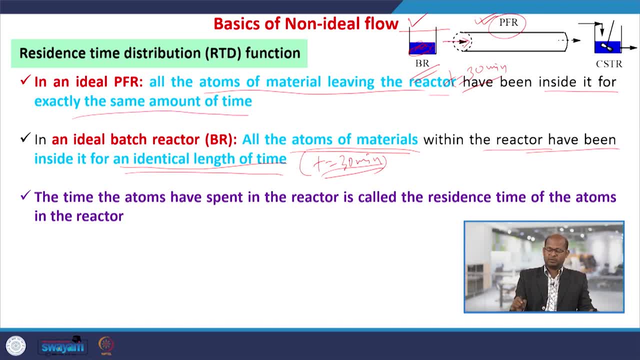 same amount of the time. see here: if there is no bypassing, no dead zone is there. so all molecules, let us say, this molecule, this is entering here and this move like this. so all molecules, whatever living along the, along the x-axis, so it is moving out from the reactor. 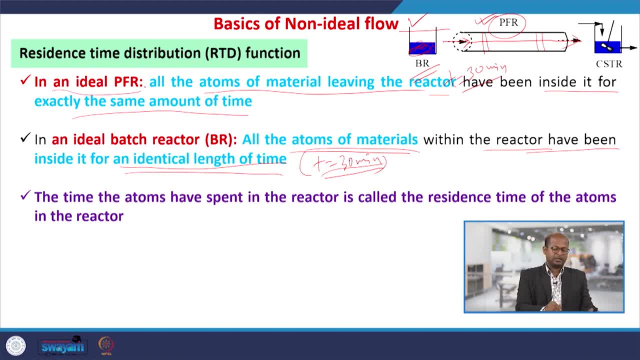 spending equal time. so then it would be also an ideal reactors. so all molecules you spend equals residence times. so then it is an ideals. in case of the chta reactors also, we are expecting here mixing: is there residence times, or the time all molecules spent should be equal, then that also. 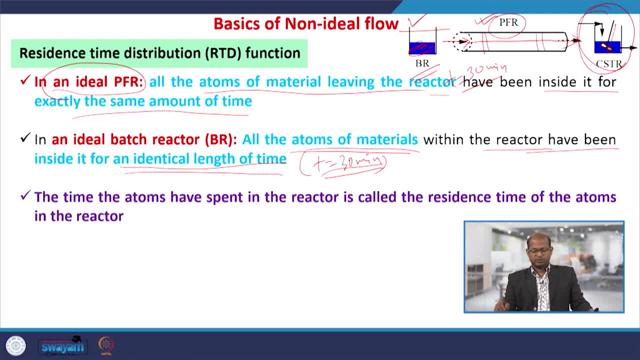 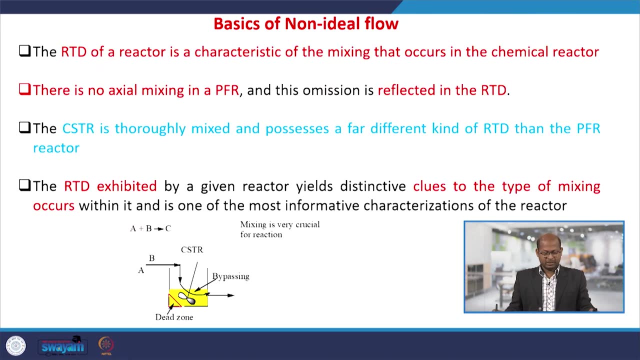 reactors should be ideals, but in real case it is not possible. some anomaly or differences we can observe. so this type of reactors is called non-ideal reactors. so in that particular reactors residence time distributions will study. so for this type reactors residence time distribution function is important. so residence time distribution. so what actually give us if rtd of 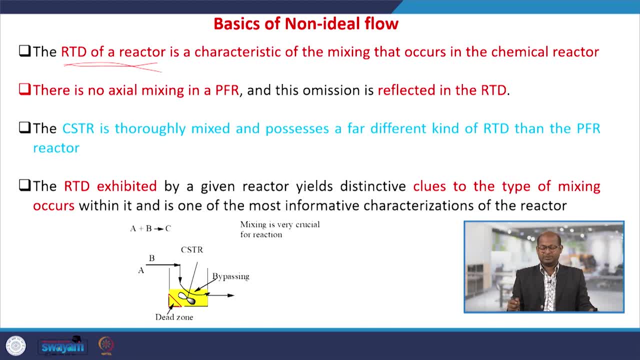 reactors. if we find out so, then it actually gives us the mixing property of that reactant. so i said reactant a and reactant b. if we do the same these reactions, if component a remain few left here, component b is leaving this way, so be spending less times bypassing. so then exact ratio will not. 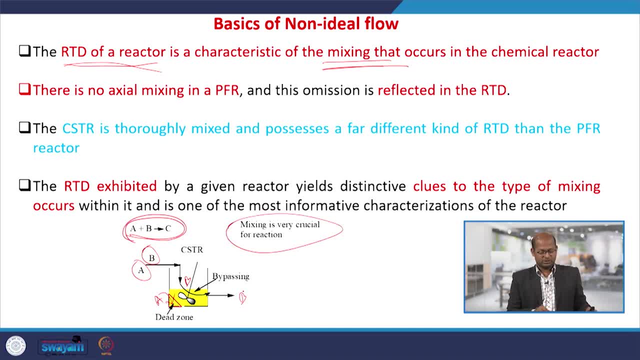 maintains, since mixing is not proper. so then, due to the non-ideal nature of the reactor, if if we exit that make here, so then would be different nature from this exit. this is the outlet of the reactors. okay, so from actually this residence time, distribution functions- if you are able to find out, you can get an idea- means whether the reactants entering so 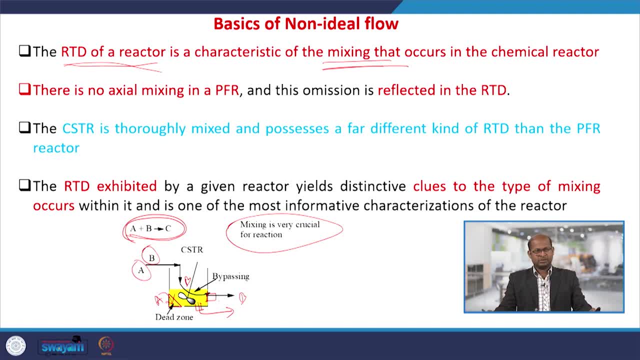 mixing is proper or not, so then by for that, so we can change the design or somehow mixing or stirring that we can change, we can put more star or somehow the some other way you can change or think about the reactor. so why it is not getting higher conversions? why? 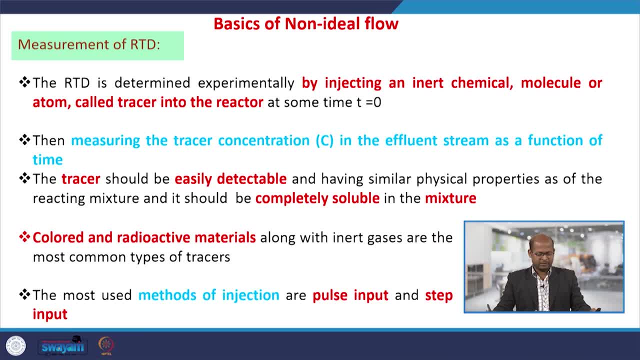 we are getting the reactant take, spending the reactors very less times. so these are the things we can find out. so to measure the rtd, or residence time distribution functions experimentally, how we can conduct so we have to inject some of the reactants. i said that reactants may be very costly, so then we cannot use that to find. 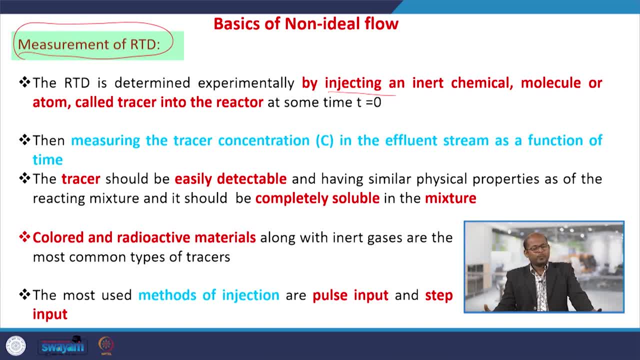 out the rtd or we can not characterize the reactors by using direct reactants, so the reactions will conduct so further that we have to use some treasures. okay, treasure materials we have to use. that may be any chemicals, very less costly, less term, price is very low. so 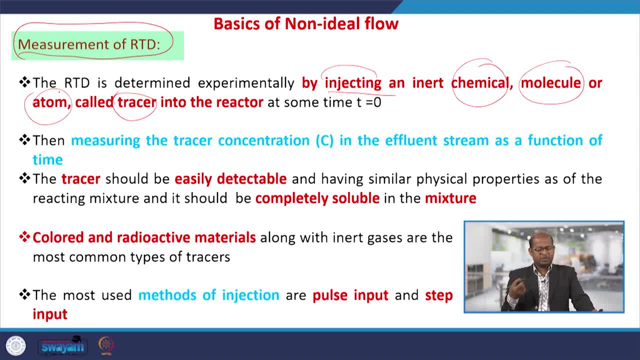 molecules we can use, atoms, radioactive materials, dye we can use that is not corrosive if it is, or NOH, whatever. These are the materials we can use, or some other things are also available: inert materials that we can use for the reactors means and find out the concentrations once it is leaving from the reactor. So these 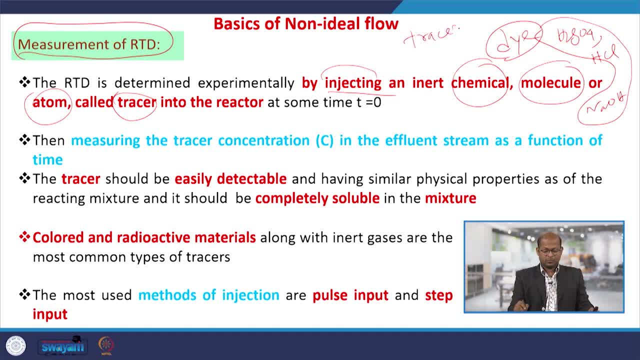 are: the component is called tracer and the tracer is called tracer or any color reductive materials also we can use And the method of suppose we have these reactors here we can inject. So here this is the feed line and normal solvent is moving and here tracer. 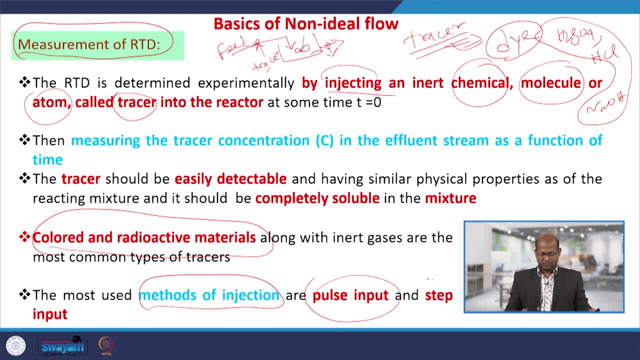 we can inject. So here this is the feed line and normal solvent is moving, and here tracer we can inject. So here this is the feed line and normal solvent is moving and here tracer we can inject. Now we will see how the injector that injections may be pulse or may be step. 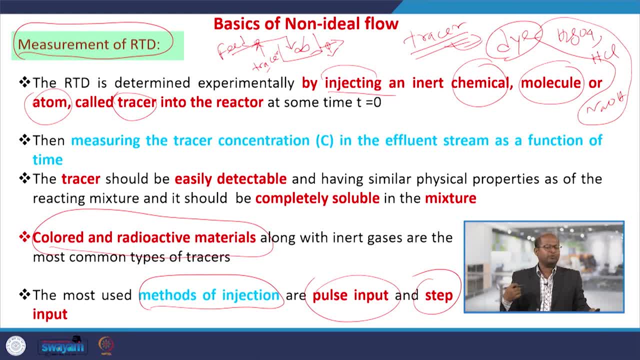 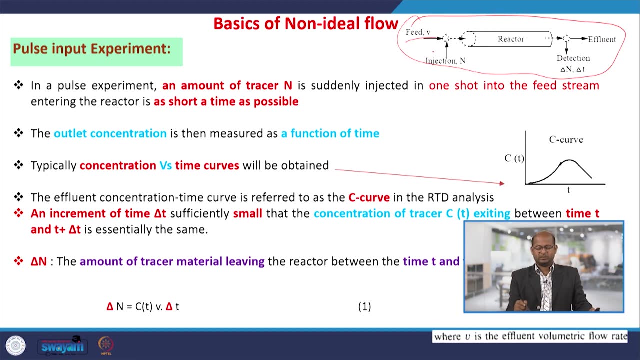 inputs. So maybe let us say, like infusion of injections in our body: 1 ml, 0.5 ml, very small quantity- we inject or infuse in our body, like that Tracer also we can infuse. This is the system. so here you can see, this is the feed lines reactant or any solvent. 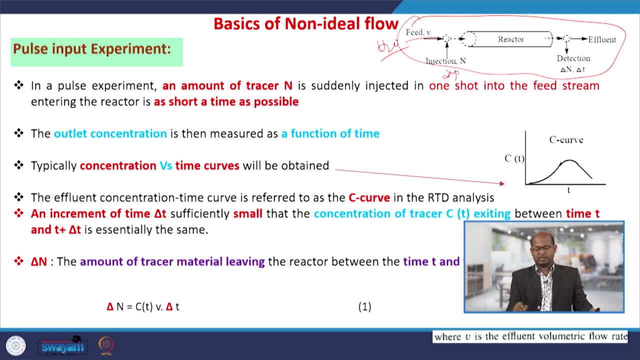 let us say water is moving and here tracer is the dye: very small quantity, 10 ml, we can inject here. it has a particular flow rate, 10 millilitre per minute. Let us say it is flowing at this particular volumetric flow rate. So from here, treasures or this dye will pass through. 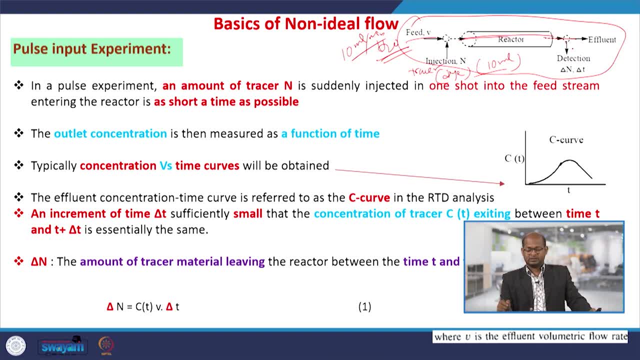 these reactors and then we can collect the effluent samples and measure the concentration of the dye at particular times. So like that, at different time, the concentrations of the dye we can measure. Like that, these are the concentrations we can measure from here, exit, and by that, if we plot this, this type of curve will come. This is called C curve. that 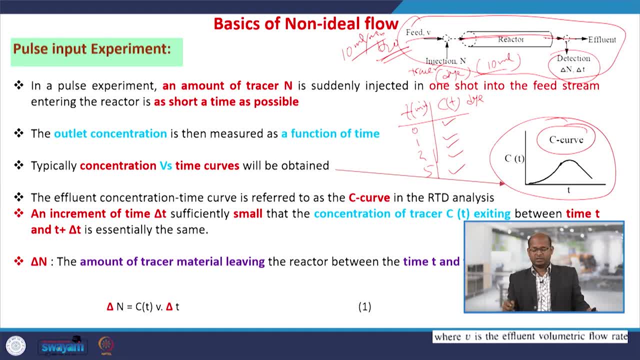 already you have studied again. you are discussing This type of treasure test. we can conduct and we can get the concentrations means changes after coming out the treasure or reactants from the outside of the reactors: 0 to 0. So what would be the concentration? So concentrations would vary. This is the treasure or dye concentration. 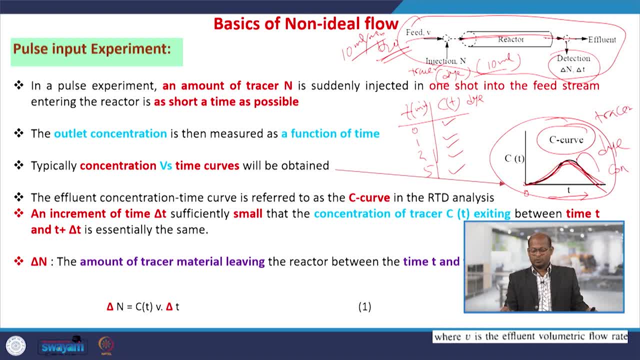 dry or treasure concentrations. These are the maximum concentration. this is the minimum concentration, So at the beginning it was the minimum, and then it is gradually increase and then drops. So this way you can find out. So now, how to get these equations means. 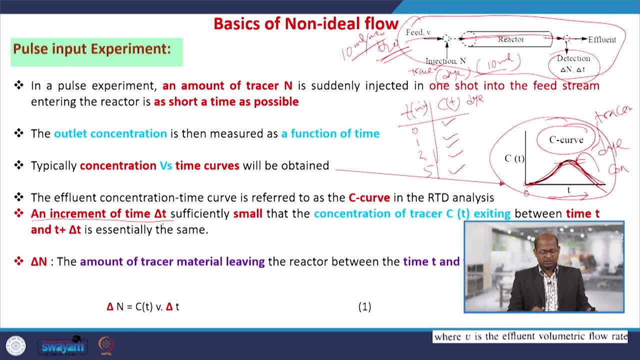 we want to develop. So let us say very small time, delta t as small. Delta t is very small time. So and concentration of the treasure from the exit. if you want to measure t time and t plus delta, t time within, that So means treasures, 10 mLs we. 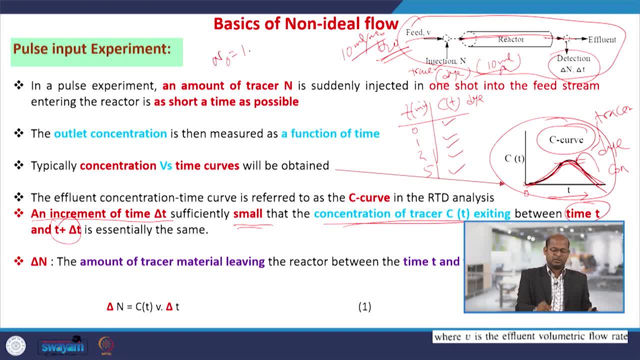 have injected 10 mLs. N0 equals to, let us say, 10 mLs that we have injected. So if you do not know how much quantity you have injected, that also from this graph also we can find out. So let us say: this is known quantity. 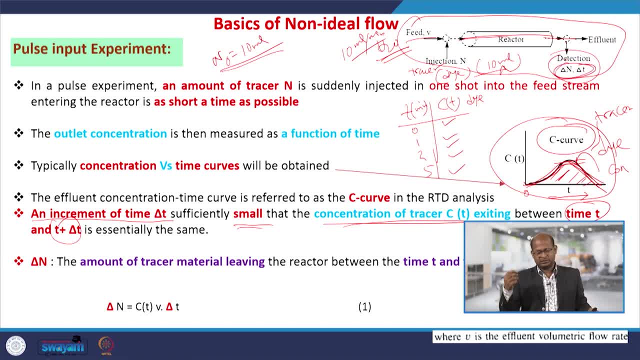 This is the after delta t times. we are getting that molecules. that is 10 mL. it was injected. delta n amount- N0 amount it was injected and we are getting delta n amount at particular delta t times. Similarly, at different times we can get the amount of the treasure leaving. 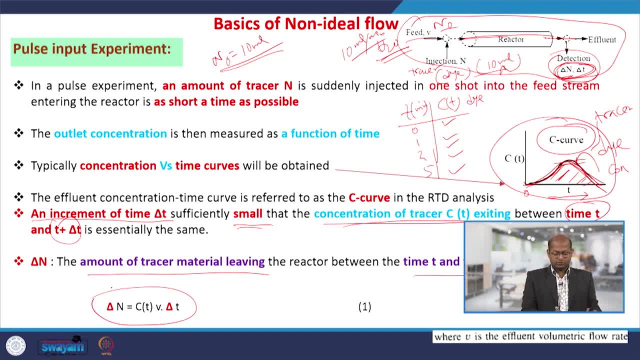 from the reactors t and t plus delta t times equals to this. So for that delta n is the fraction of N0.. So delta n amount it may be delta n. maybe let say 0.5n, So you can 0.5 ml at delta T may be 10 minutes. we are getting delta T equals to 10 minutes. So 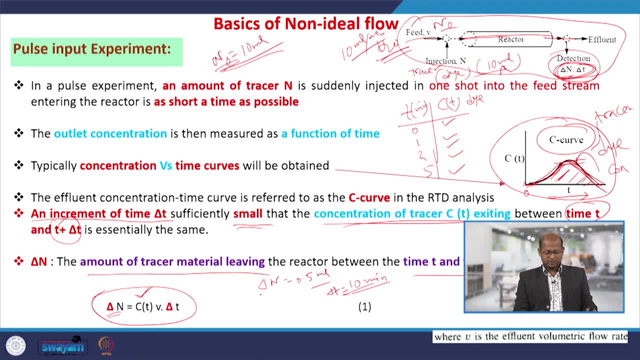 this is the concentrations we can measure at that particular time. This is the N0, that is, the delta N amount of the quantity of the material in terms of milliliter grams or kg we can find out. This is the volumetric flow rates we know. So then, delta N equals: 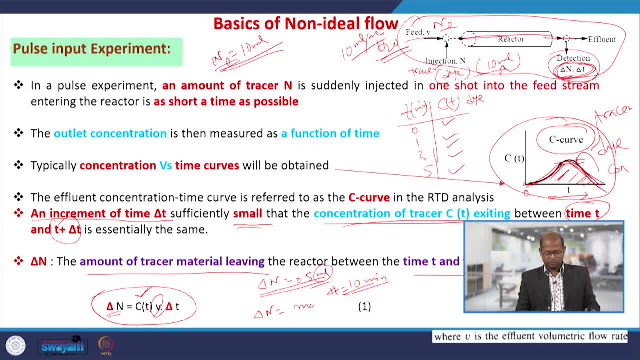 to the amount of the material. that is equals to Ct. equals to mole per dmq. Volumetric flow rate is as unit dmq per unit time, minutes, let us say, into delta T equals to minutes. So we can this that amount of the moles leaving from the reactor. So we can easily find out. 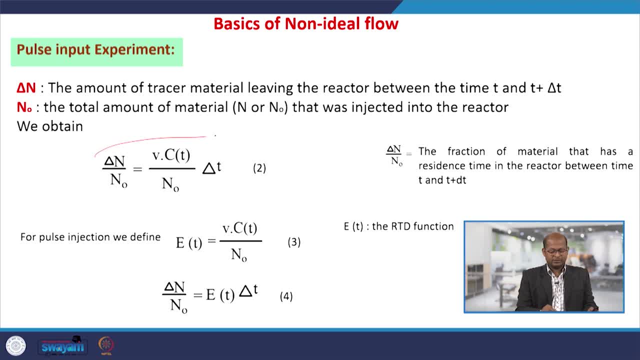 using this equation 1.. Now if we divided these equations both side, left side and right hand side. equation 1 if we divide with N0.. N0 is the initially the amount we have taken. So delta T equals to 10 ml, and after a particular time. So let us say 0.5 ml, or in terms of: 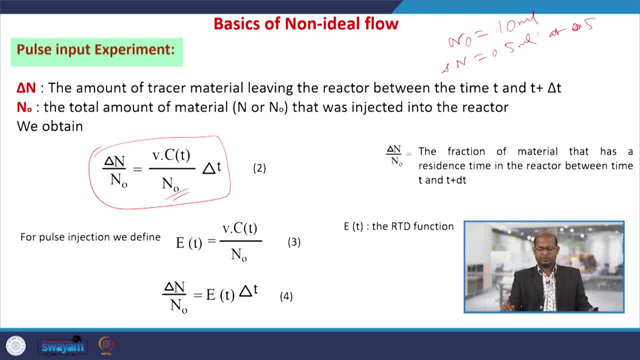 kg at 0.5 or 5 minutes, we are getting delta. T equals to 5 minutes intervals. we are getting. So, if we divided, left hand side N0, right hand side also N0.. So then we will get delta. 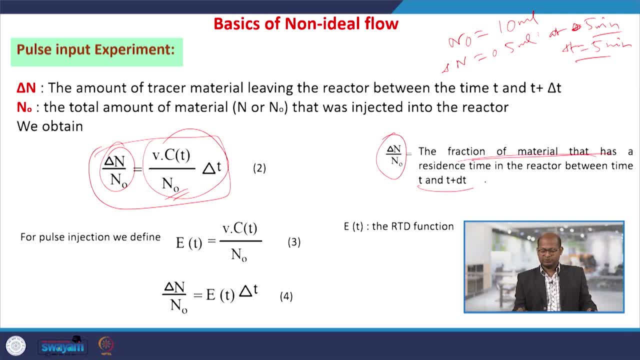 N by N0 is the fraction of material that leaves in the reactor within this time: T and T plus delta T within this delta D fraction. So delta N by N0 is the fraction of material that leaves in the reactor within this time. 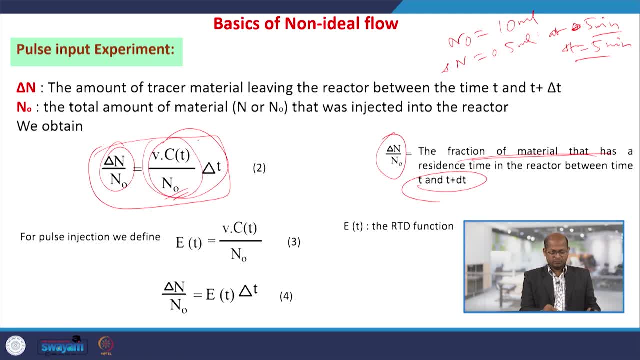 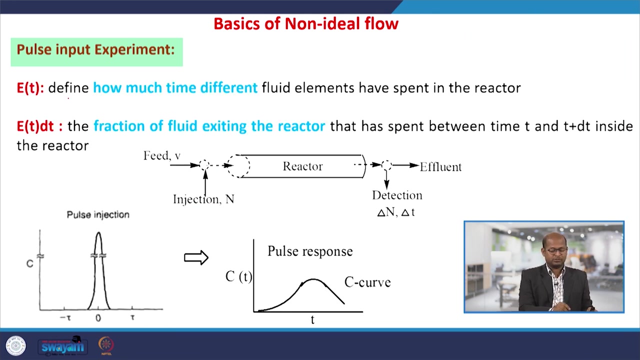 So there is E, t is the residence time distribution function, So how much time different fluid elements have been spent inside of the reactor. So E, t, that is the residence time distribution function. So what does it signify? It indicates actually how much time it is spent, means we: 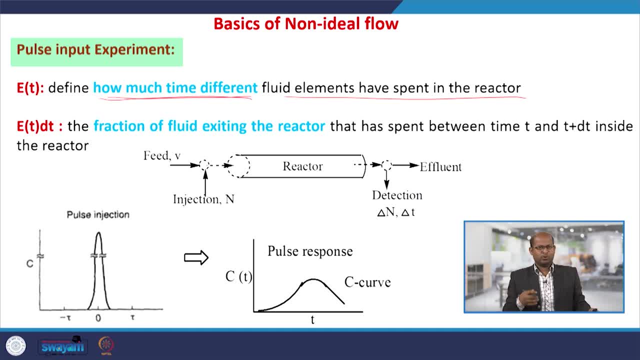 have 10 ml injected, So in 10 ml all molecules. if it is spent equal times, then that is very good. if it is not, if all molecules does not spend equal residence time inside of the reactor, then nature would be different. So from that we can get. 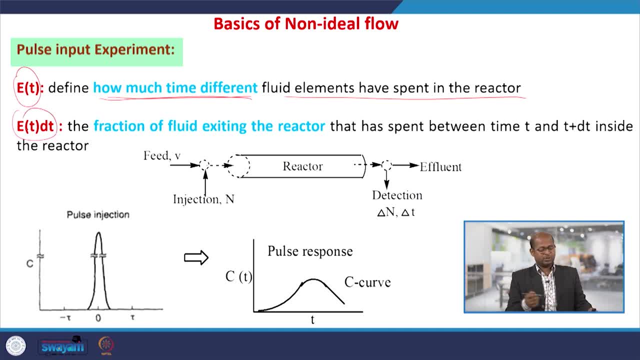 So E, t has units. that is time inverse. if you multiply with the time, that is the fraction of material that is living within that stipulated time, t, and t plus dt within that reactors. So this is the injection, this is the concentration of the tracer or dye that is used for the 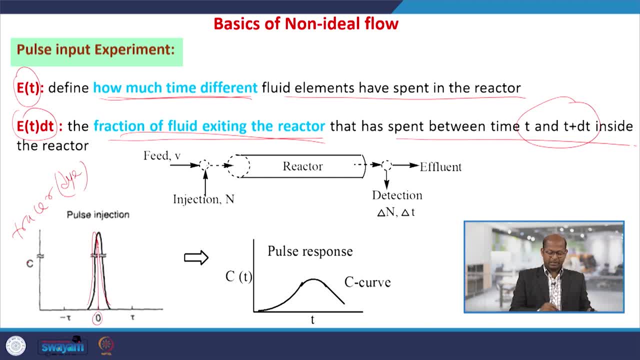 injection that we have taken, and so this is the 0 means ideally, means infusion. So whenever concentration of the tracer 0 times So means minus tau, plus tau, Let us say this. so actually this time is this means concentrations whenever we inject inside. 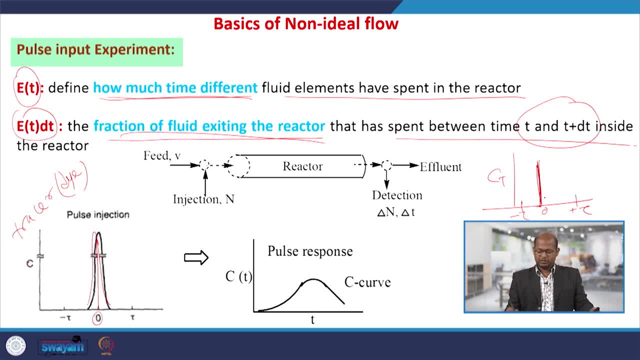 of our body, any injection. So then it should take fraction of times, less than very low times. fraction of times means less than 0 second. that should be, but this is the ideal, but in real case this is the real means injections or pulse injection- that whatever we do, it takes some. 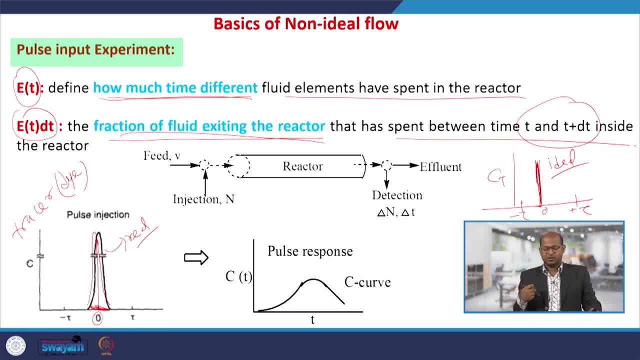 times means one second maybe if we infuse anythings in our body or this fluid system. so injections it takes some times. so ideally it should be a lines, but in real case it should be like this: so sudden jump of concentration of reactants or treasure that is injecting. 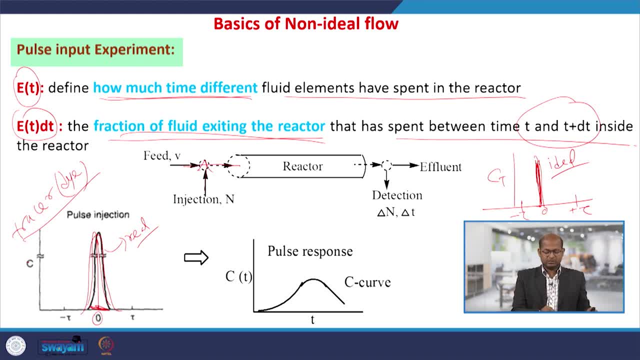 inside of the reactor. so here initially is when there was no treasure infusion. it was zero when suddenly injected the treasure inside of that line. so sudden jump of the concentration should be. this means initially it was zero, sudden jump and after that distribution of the treasure should be here that spins inside of the reactors and then it leaves. 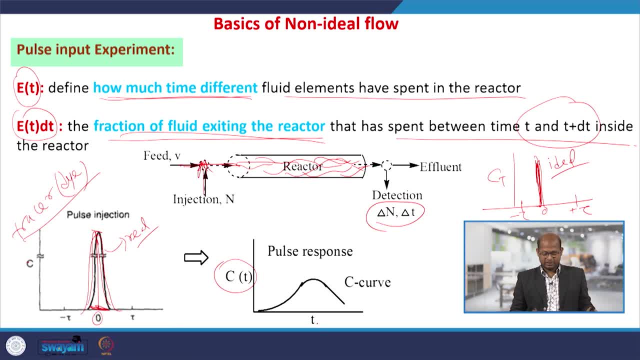 so if we know this, then concentration versus times we can plot. and it would be like this: this is the pulse response, this is pulse injections and this is pulse response. this is pulse injection, this is pulse response. so from the pulse response we can get c curves. 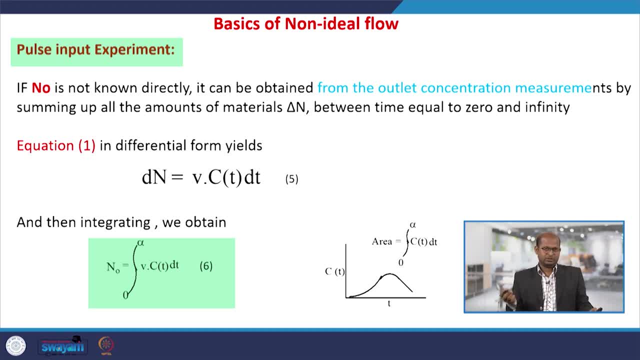 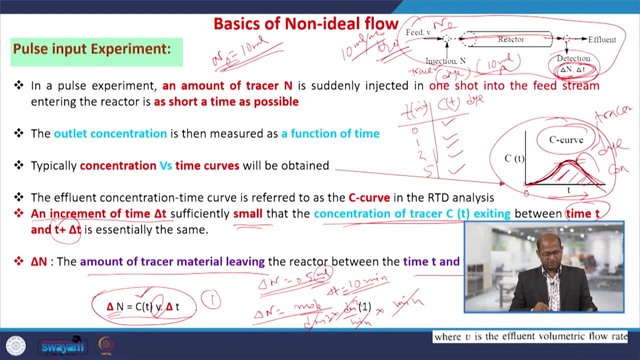 so now a n 0 is known. if it is known, it is very good. if it is not known, also, we can find out using some equations. so now equations. once was in terms of this equation one. this was the equation one. this was in terms of differential forms. 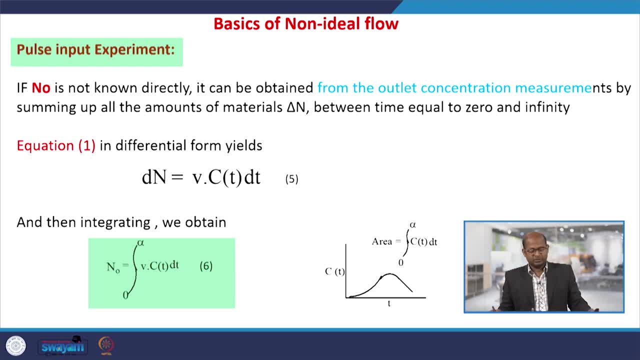 so delta form. so now, if we express in terms of differential, differential forms, this equation, once we can write, this means: delta n was there equals to v c, t into delta t was there. we are expressing this equation in terms of differential form. now, if we integrate zero to infinite times, 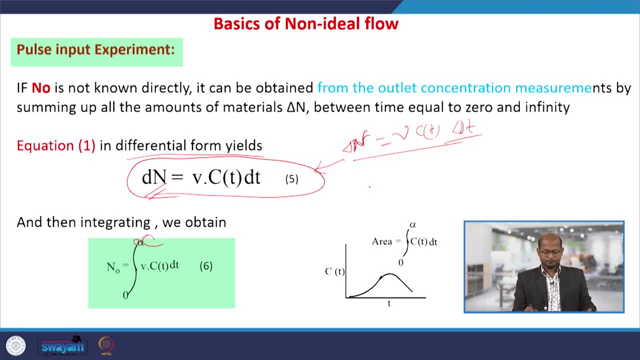 so then in the left hand side, d, n, zero to infinites. if we integrate that would be equals to n, zero. so in the right hand side integration is there: v, c, t, dt, so equation six. so if we concentration and time, 63 curves is there. if you integrate and find out the area, total area. 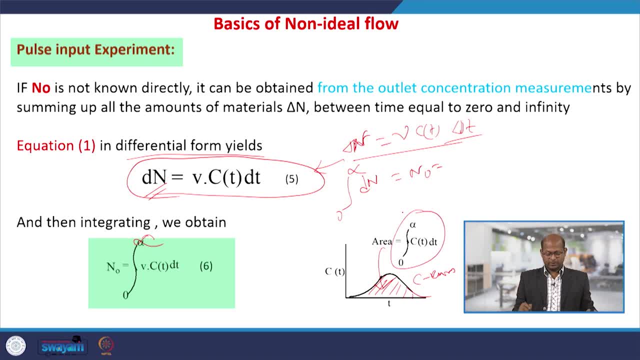 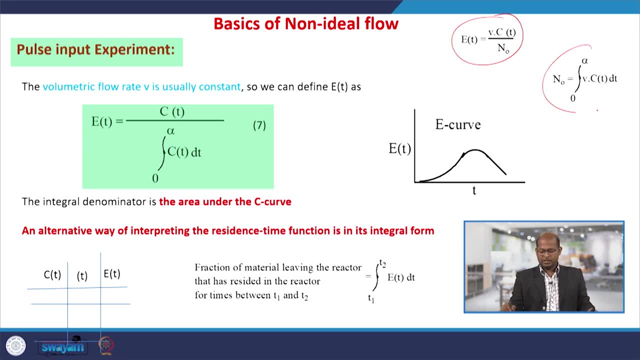 that is this, so now volumetric flow rates. so it equals to v c terms. so if we integrate d, n, hemos dos n0. so so now volumetric flow rate e, t equals to pitch heart is there, or rp. so, and now volumetric flow rate is Ct by N0, N0. is this, So N0 equals to this. from this equation 1 or this equations: 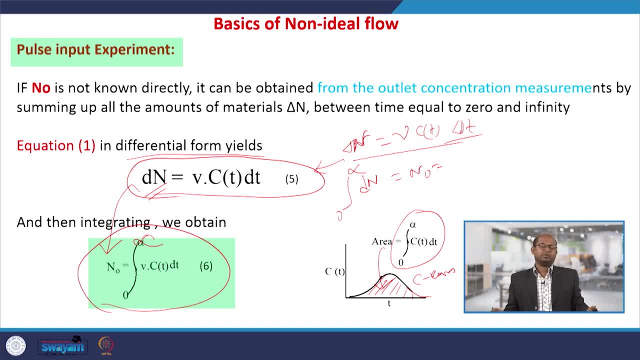 after integrations: 0 to infinite time. the infinite times may be total, stipulated times that may be 1 or 2 hours required to come out all the reactants from that reactors or all the tracer from the reactor. So that way we can find out the total N0 amount of. 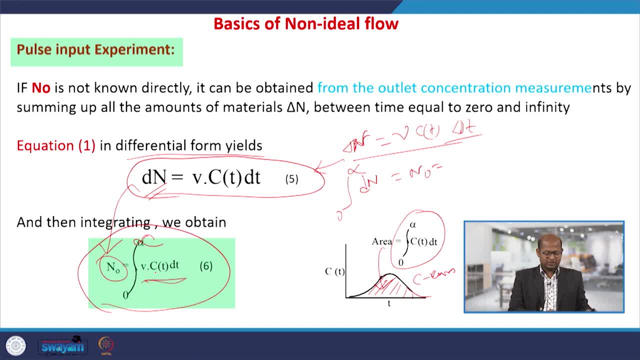 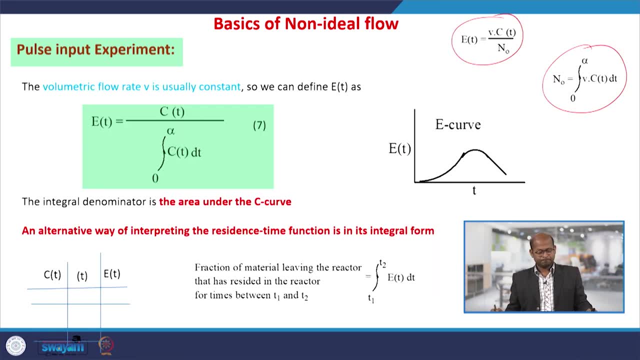 the tracer that was injected, So by integration. Ct is known. V0 is the constant. if V0 is the constant, so if we know so, then say N0 value, we can find out. So now, volumetric fluid is usually constant, V equals to V0, so that now Et equals to this. 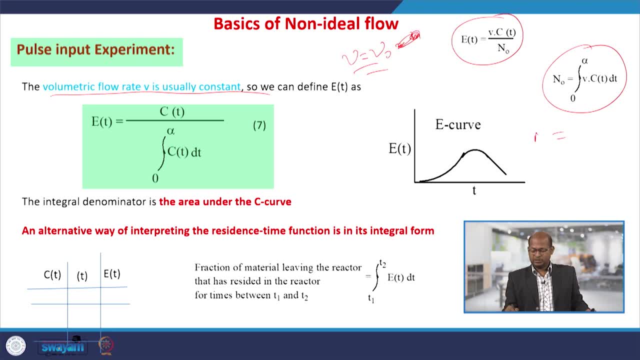 if V0 is constant, V equals to V0, so then N0, we can write V0. 0 to infinite Ct, Dt we can write. So now this N0, if I substitute here, so V equals to V0, V0 equals to V0,. 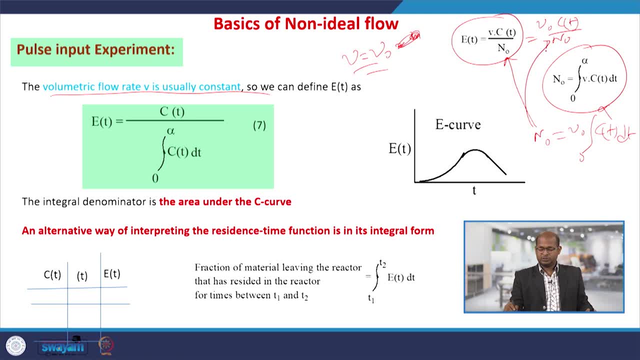 Ct by N0.. So N0 substituting here V0 we have. so after simplifications we can get this: Et equals to this way: Ct by 0 to infinite Ct, Dt. this way we can express So this area. 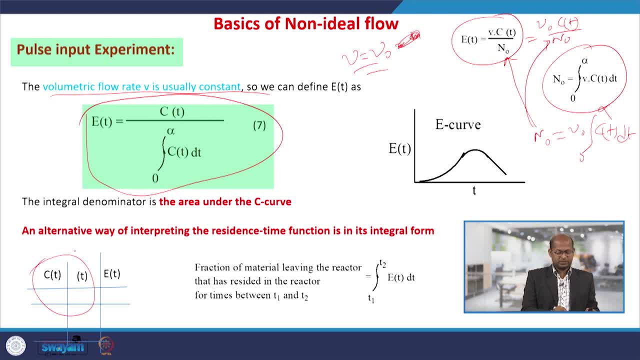 under the curves we can get. so means from the experiment Ct concentration at different times we can find out. and once we know then this Ct value we can put it here and Et value we have to find out. So we have to integrate. this means from the C curve, this part we can get, so then we 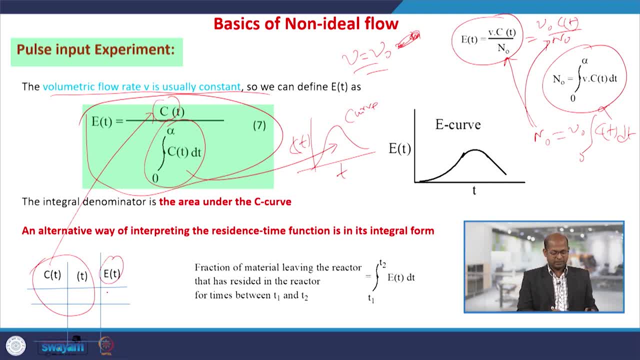 have to divide Ct with this. then we will get Et. So this way we can. individual times means 0, means T equals to 0,, 1,, 2, 3, concentration: from the experiment we can get corresponding Et value also. we can find out so once we know. 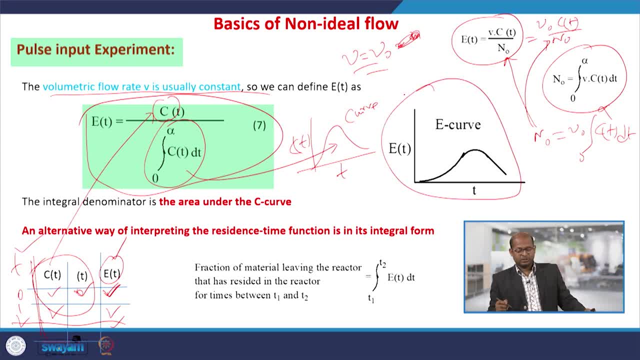 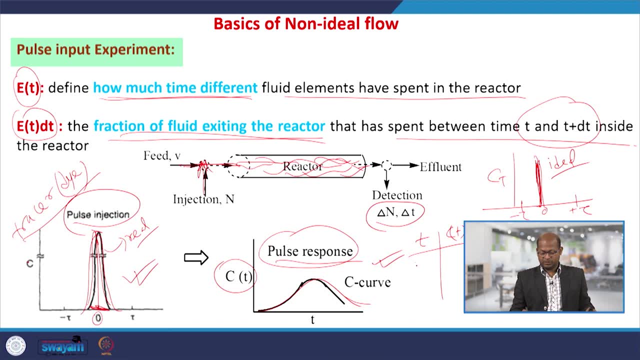 So E, t and T, if we plot, then E curves we will get. So how to get E curves that we know. how to get C curves, that we know. So if we times concentration of the effluent concentrations we can know. so if we plot, then C curves we can get and E curves we have. 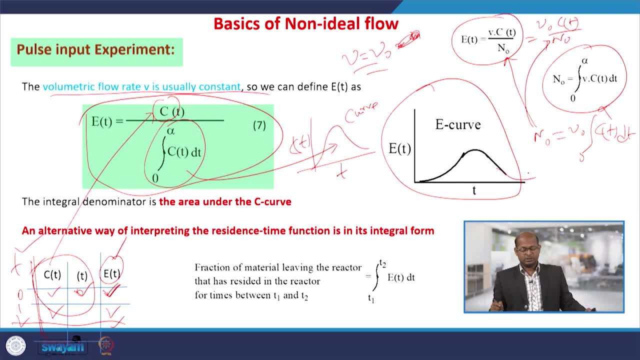 to find out. So, similarly, if we know, then E curves also, we can get C curves, E curves And see here at any times. within that, T equals to E, total time is 0 to 20.. So if, let us. 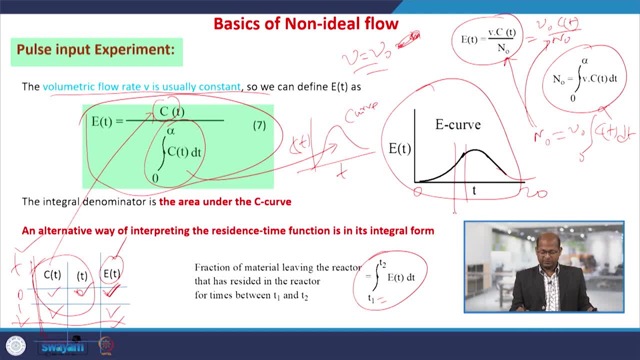 say, within that stipulated times, how much fraction of material living: 5 minute to 7 minutes. so then T1 equals to 5, T2 equals to 7 minutes. So if we know Et, dt, so then that way fraction of material living within that 5 to 7 minutes, that easily we can find. 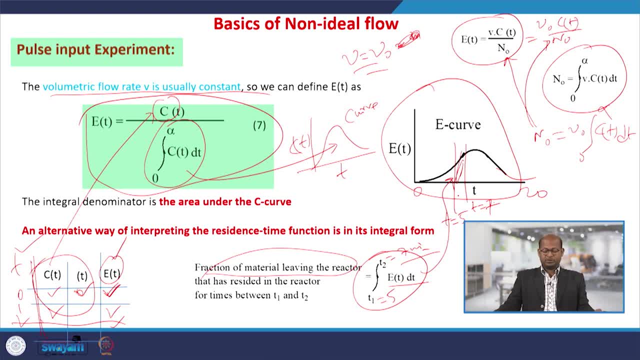 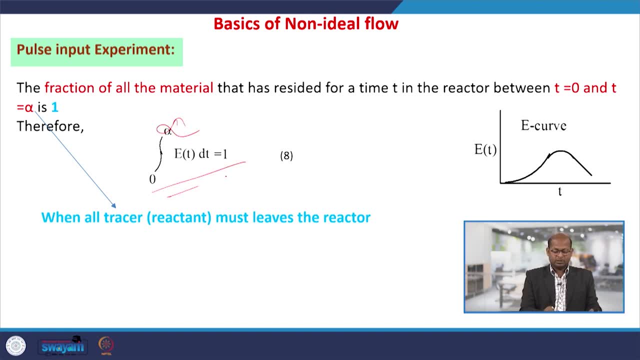 out using this integration procedure or this way, if we know the Et value, So total 0 to infinite Et, that would be 1.. 1. Means 1, why it is coming. this is equals to N0 by N, So N0 by N0.. So therefore it. 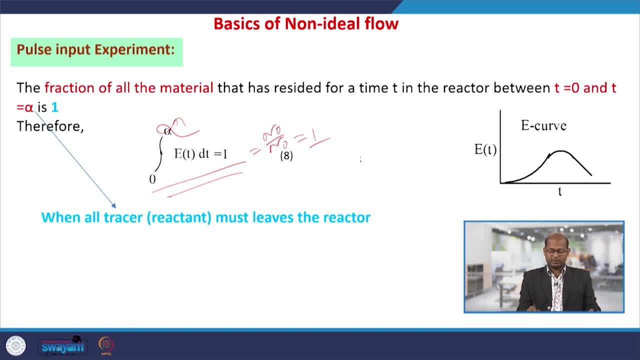 is coming 1.. So N0, actually the fraction of material that is living, N by N0.. So N1 plus N2 plus N3, plus like that it is coming N0 by N0. is this N0? is this N1 plus N2? summation? 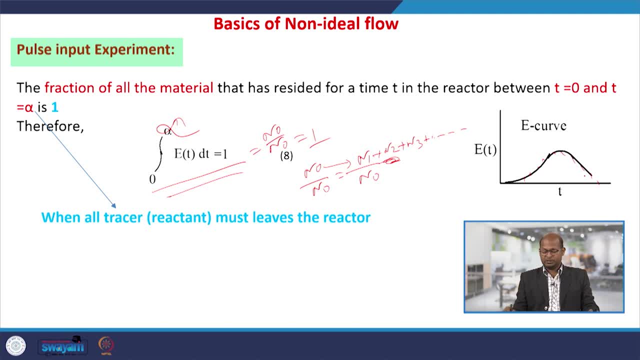 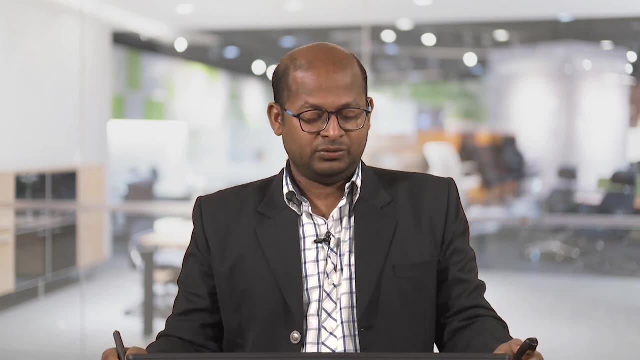 of these molecules that is living at this particular point. if we sum up, then total summation of molecules that was injected that we will get. Therefore it is coming 1.. So thank you. So today, up to this means what we have studied so far, means how to means 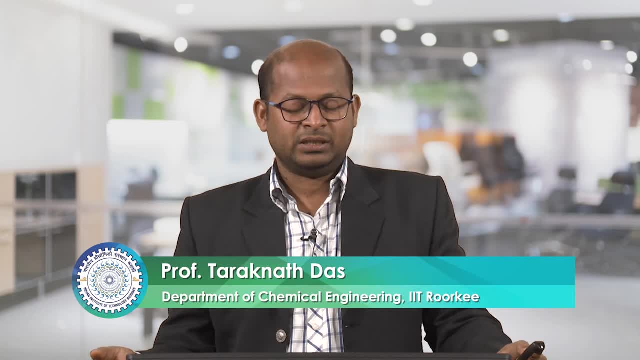 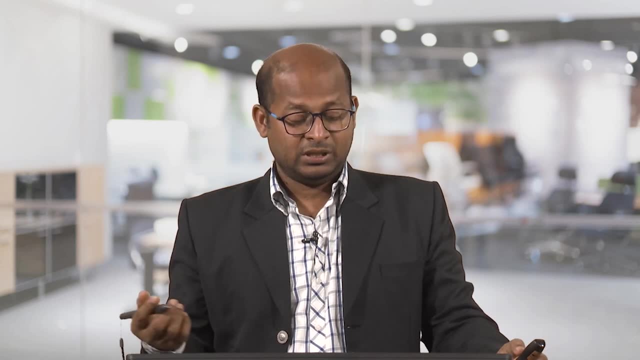 different reactors, what are the different problems, what is called ideal reactors, what is called non-ideal reactors, and how to find out the what is called residence time distribution functions. and how to find C curves, how to get E curves. So thank you.